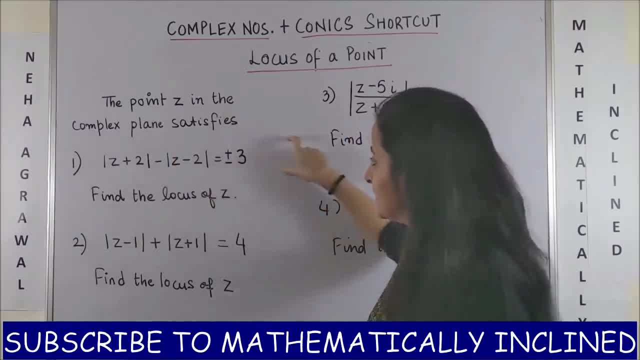 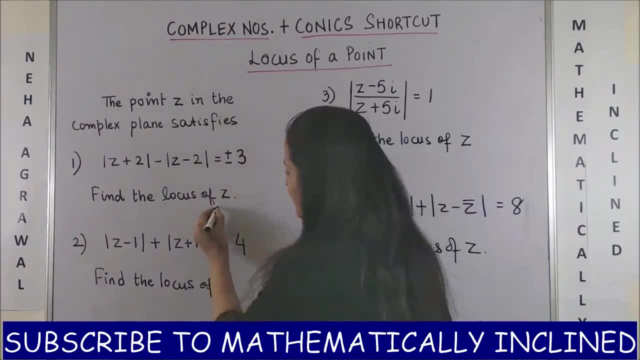 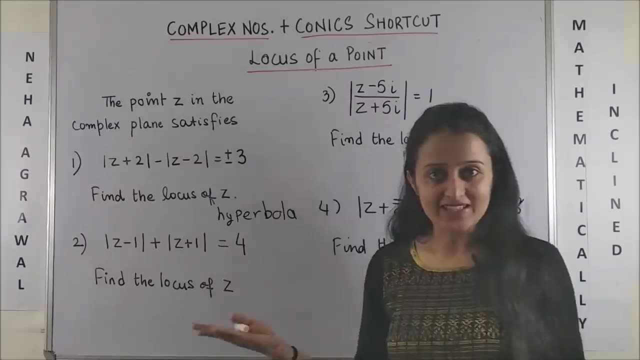 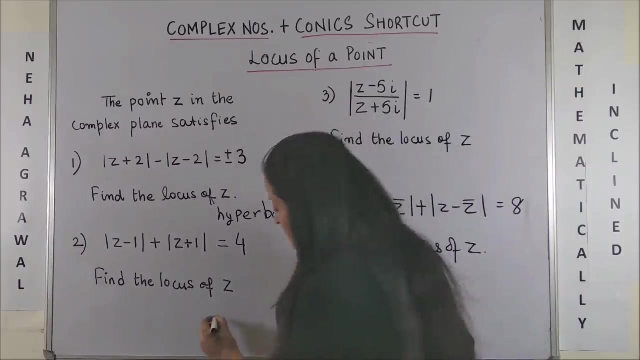 Argon plane or the Gaussian plane satisfies this condition, this complex equation. then find the locus of Z. The answer should be: it would make a hyperbola. That's it. The second one, the same question, and this time this is the equation: The locus should be: 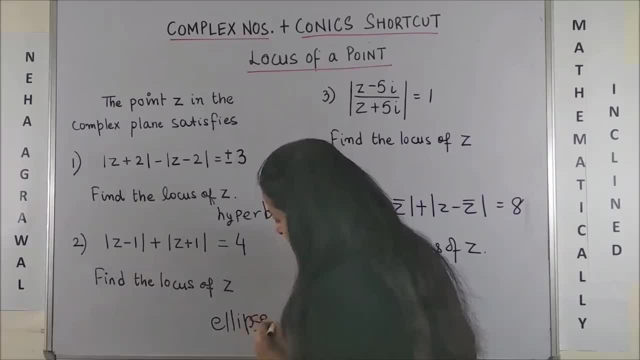 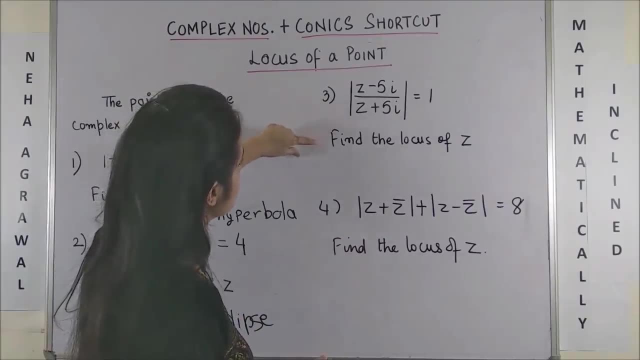 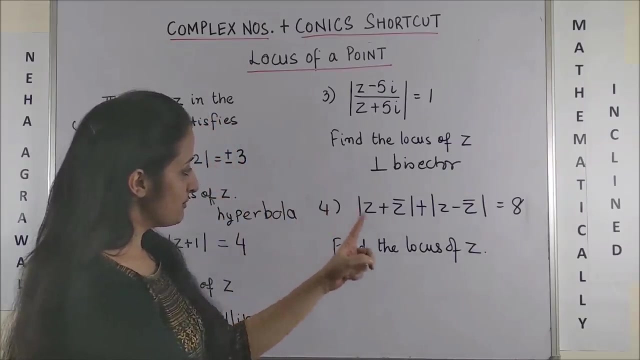 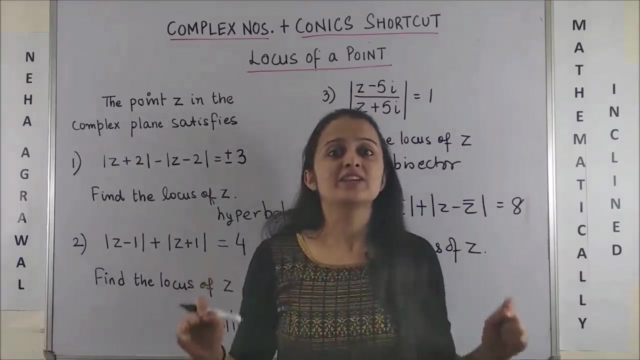 an ellipse. Yes, coming to this one, this tells us. here, the locus should be the perpendicular bisector between the points joining minus 5 iota and 5 iota. And for the fourth one, the locus should be simply a square. Yes, it is this symbol to identify. Stay tuned till the end of. 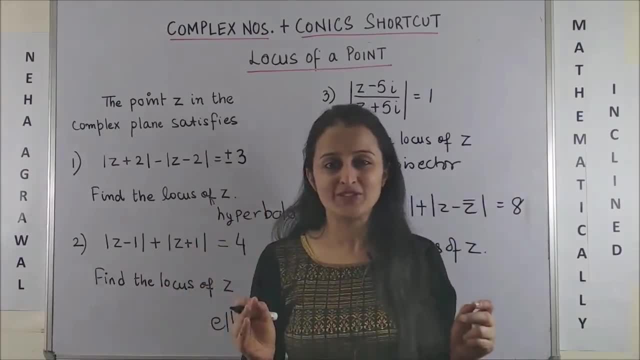 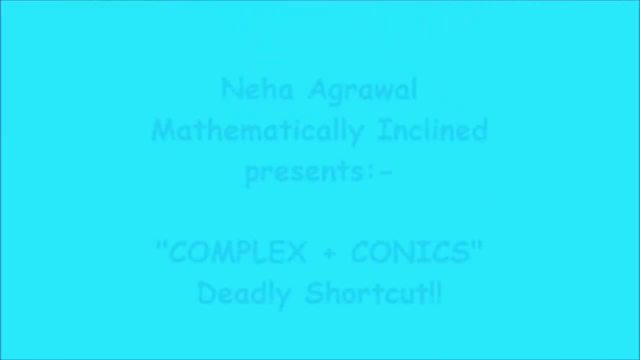 this video, as I discuss a lot of questions and the level of the questions keeps going higher and higher. So here's the magic for each one of you. So suppose you are given to a different class. Which class? The first one? The second one? 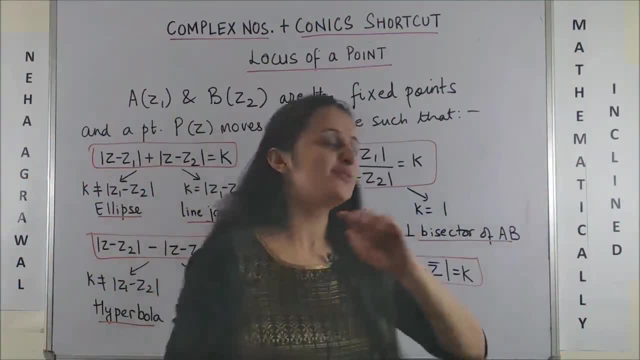 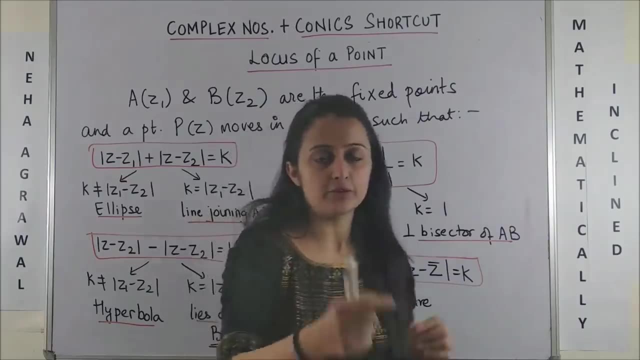 The third one, The fourth one, The sixth one, The sixth one, The seventh one And the sixth one, The fifth one And the sixth one And the seventh one, The sixth one, given two complex points, z1 and z2. now, in place of these z1 and z2, you could 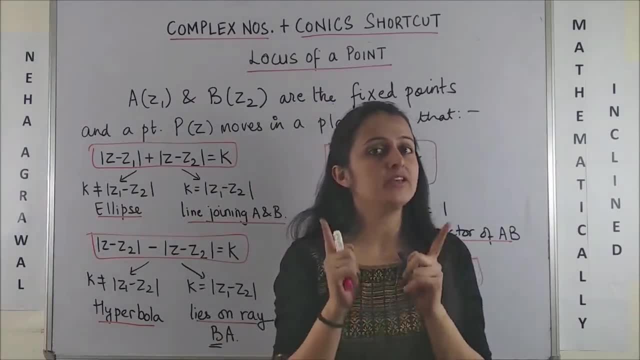 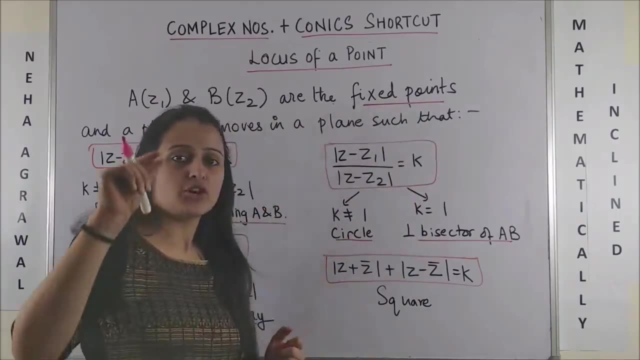 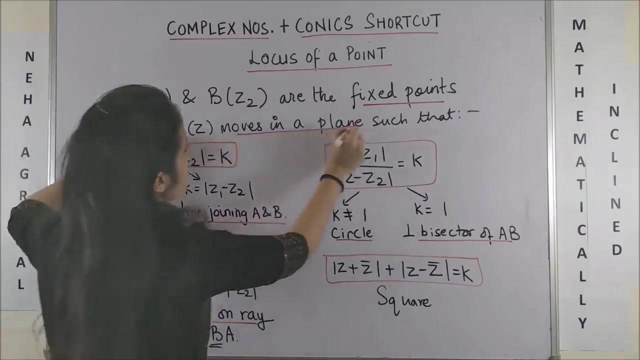 also have basic real numbers, because you know, every real number can be expressed as a complex number. so they would be given to be the fixed point. so, in short, there would be a constant value allotted to them and a point, P, moves in a plane such that it satisfies a certain condition. you have to find locus of this. 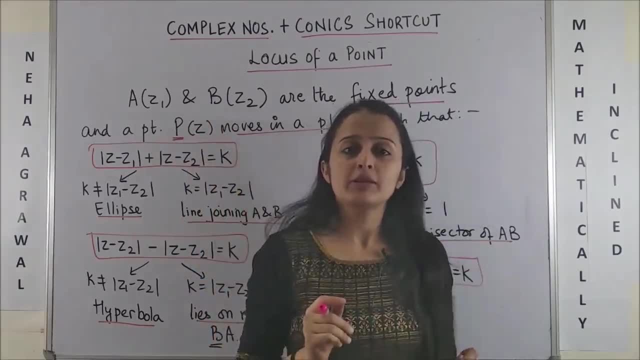 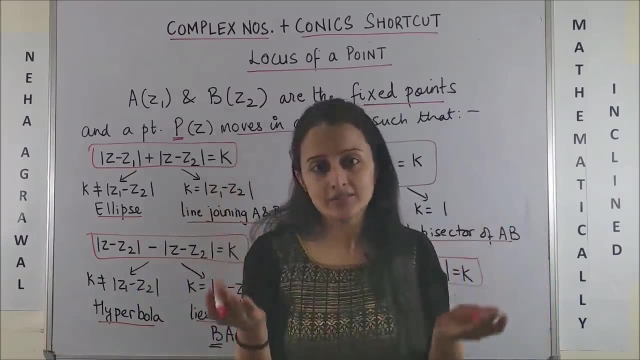 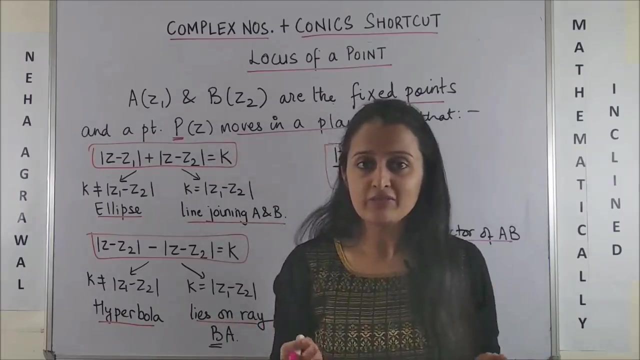 point P or locus of this Z. now, what do I mean by locus? that, under the given conditions, when my point P moves, it traces a certain path, it traces a certain curve. which curve is it is for you to identify. you might feel they are very overwhelming, or, in short, they'll be very difficult to remember. but trust me, 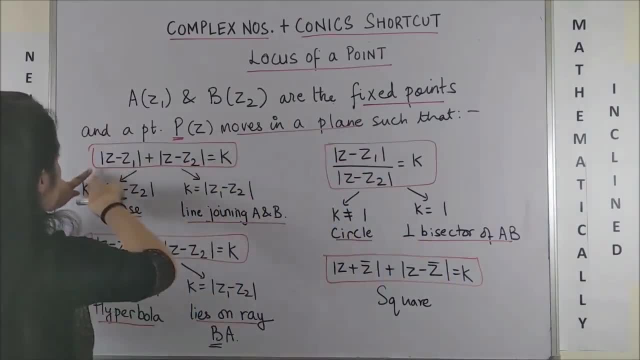 that is not the case. so each time you come across this form, mod z minus z1 and you're looking for the symbol plus, mod z minus z2 is equal to some constant. all you need to do is mentally check: is this constant coming out to be equal to z1 minus z2? if your 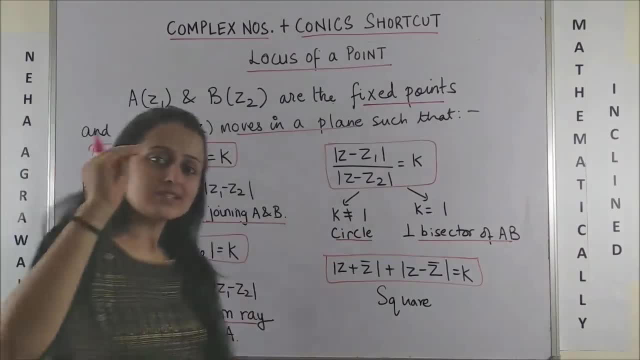 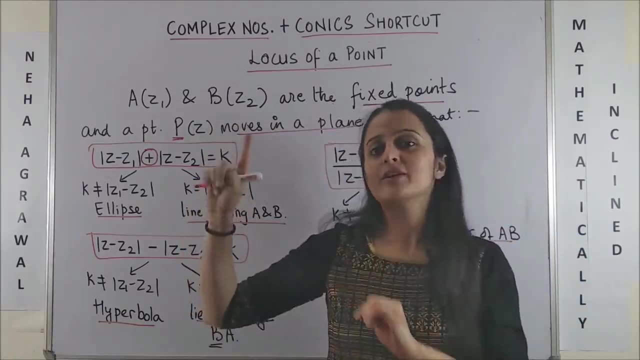 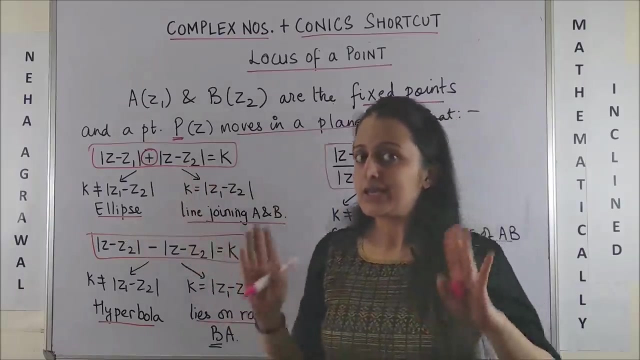 answer is no, then it's a simple ellipse, so very similar to your equation of an ellipse which was x square by a square plus y square by b, squared equal to one. so if K is not equal to there difference that it's simply an ellipse. and in case it is equal to this, then 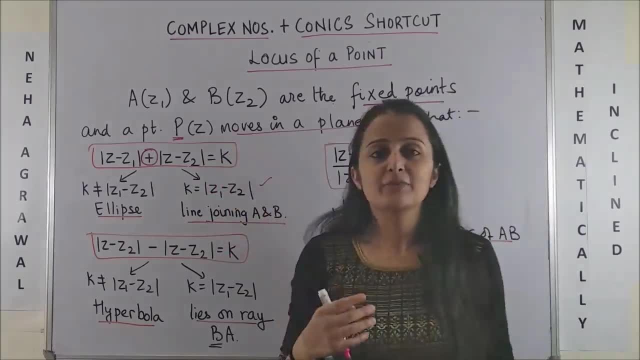 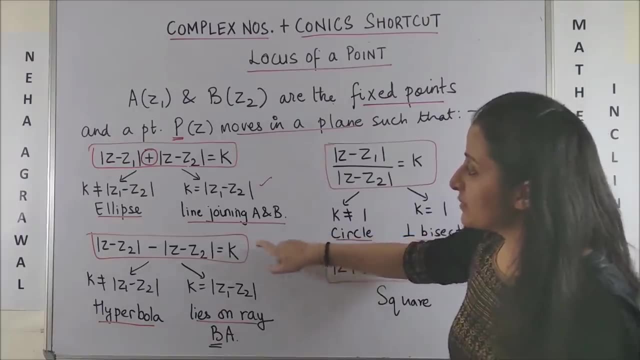 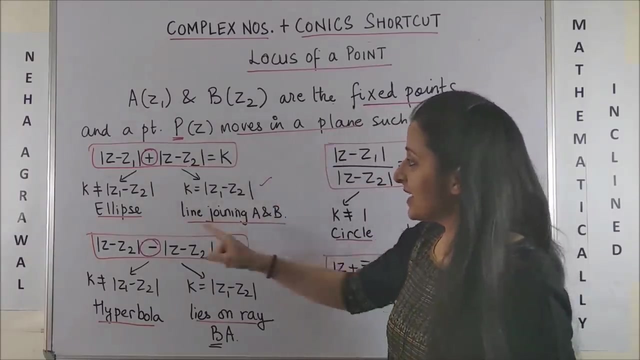 this P would simply lie on the line segment joining these points a and b. very simple to remember. likewise the next equation, very similar, but in place of plus you have a minus sign in between. then in that case, again the same logic: % G993.. pegar 0.0GSm. if k turns into z0, if zおい aspect becomes zero, then that 느vung ællaw midХŷa. 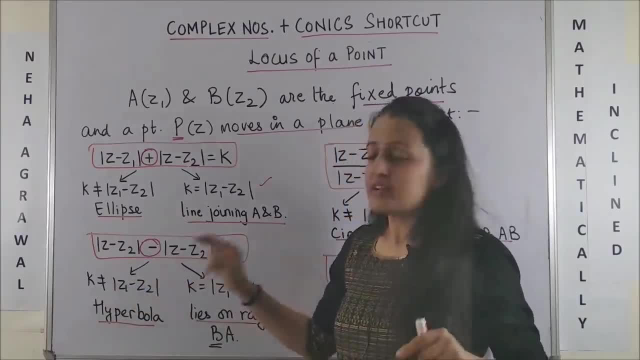 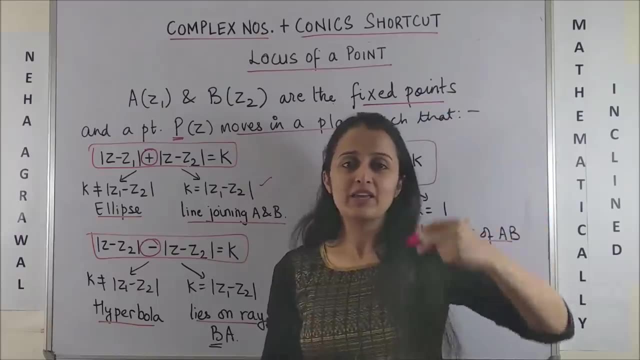 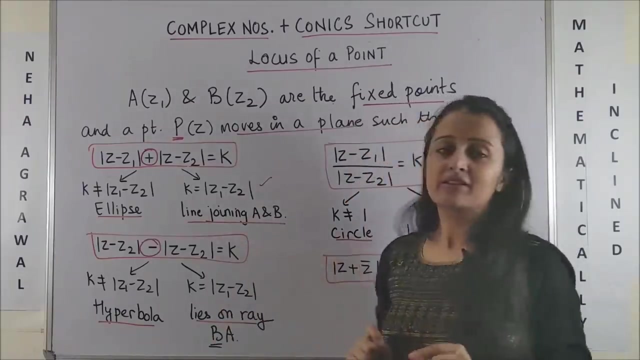 out to be. if k is not equal to z1 minus z2, then it's simply a hyperbola, Very similar to your equation of hyperbola, which was x square by a square minus y square by b, square equal to 1. and in case your k is equal to z1 minus z2, then this p lies on the ray ba. 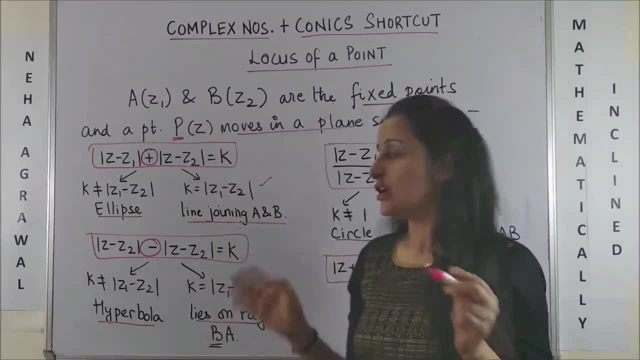 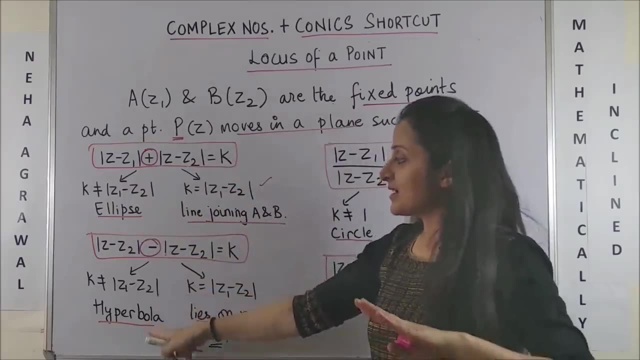 Ba means beginning from b and moving towards a. So you basically have to remember: for plus it's an ellipse, if it is not equal for minus, it's a hyperbola, if it's not equal for plus, if they are equal, it's simply on the line segment joining ab and this is on the ray joining the. 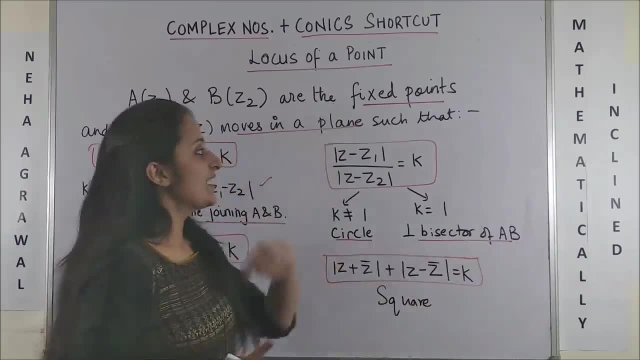 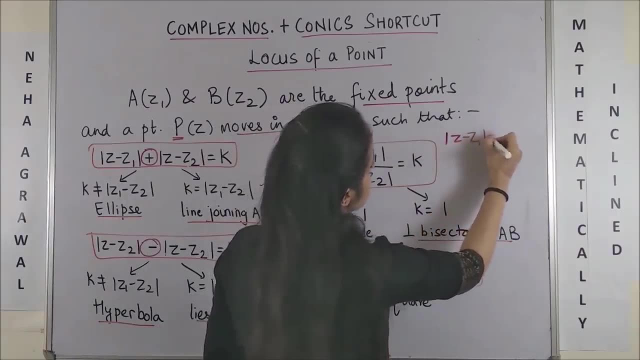 ulta, which is ba. So on this side I have, if you come across the same thing, in place of this you could also be given: mod z minus z1 is equal to k times mod z minus z2.. So it could be in the ratio. 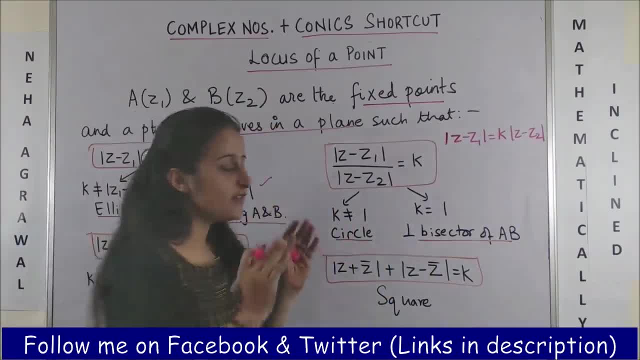 form, or mod z minus z2, is equal to k times mod z minus z2.. So it could be in the ratio form or may be this form- then in that case, if your k is equal to 1- in short, I am trying to say if your 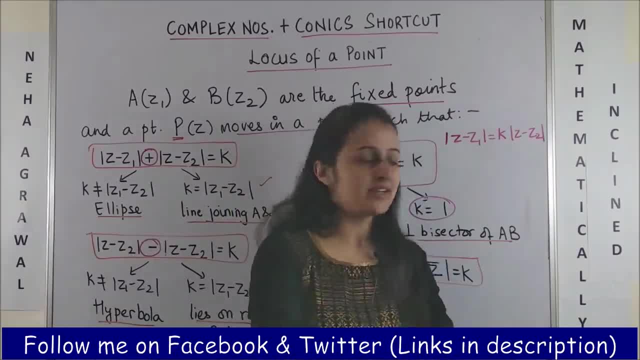 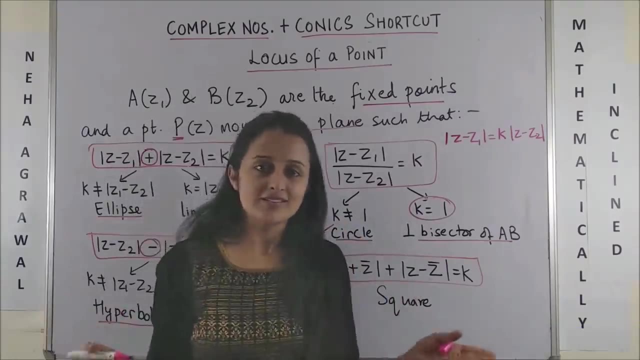 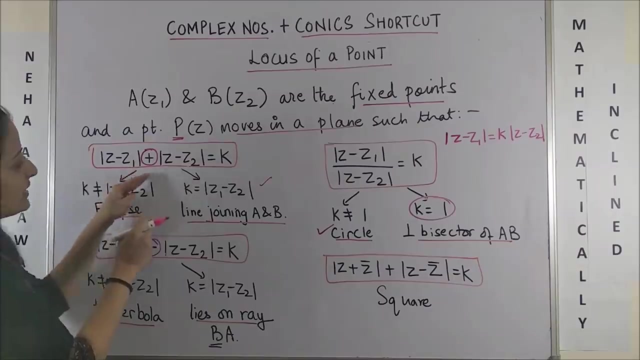 mod of z-z1 is the same as mod of z-z2, then simply, your p lies on the perpendicular bisector of ab. yes, and in case k is not equal to 1, then in that case it is simply a circle. Lastly, this is a very special case that you know. it's very similar to this ellipse equation, but in 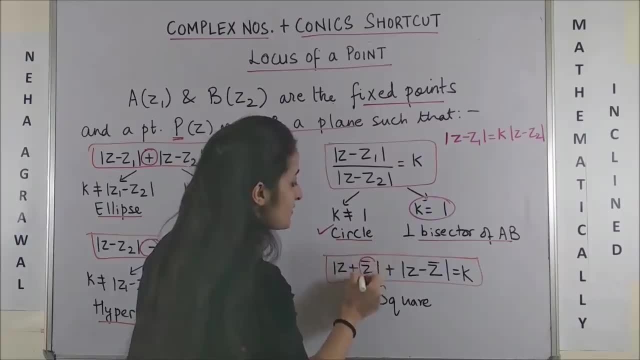 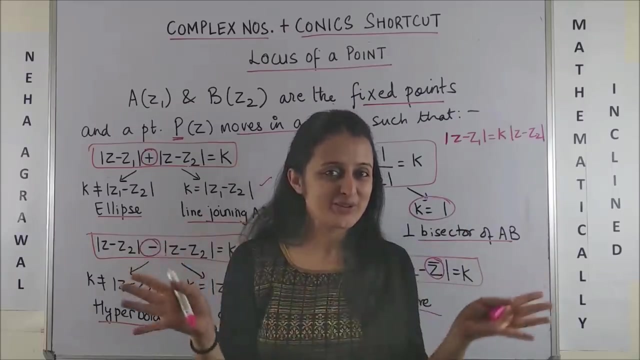 place 1, but in place of z1 and z2 you specifically have the conjugate equal to some k, then in that case it has to be a square. Make a note of all these very carefully and then, trust me, all the questions would become bachcho ka khel. 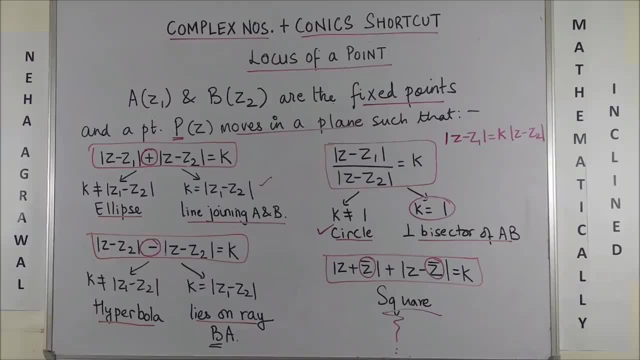 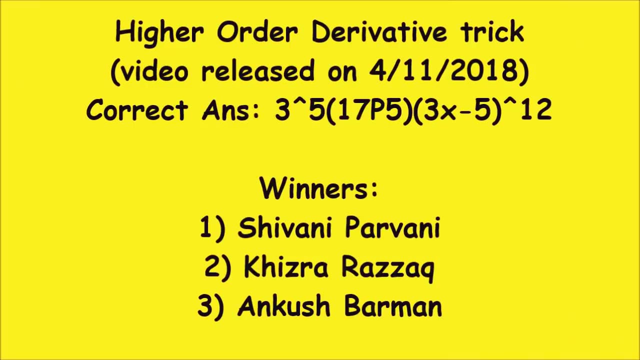 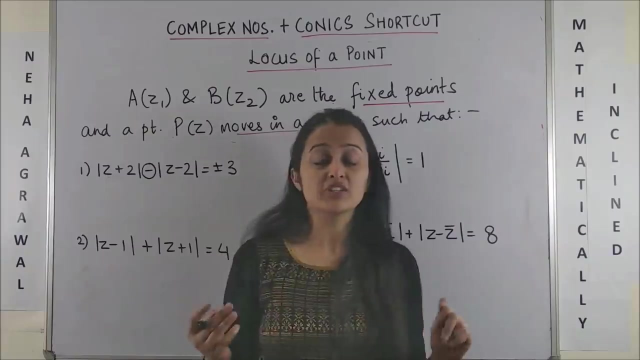 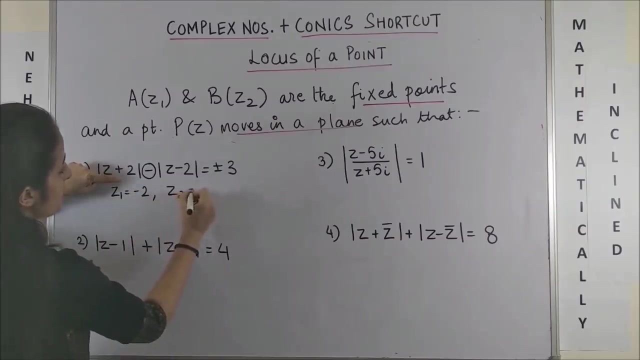 When you look at the first question, since there is a negative sign in between, the first expectation is it could be a hyperbola. So here, if you realize the form, your z1 is minus 2 and your z2 is plus 2. mod of z1 minus z2 is equal to minus 2 minus. 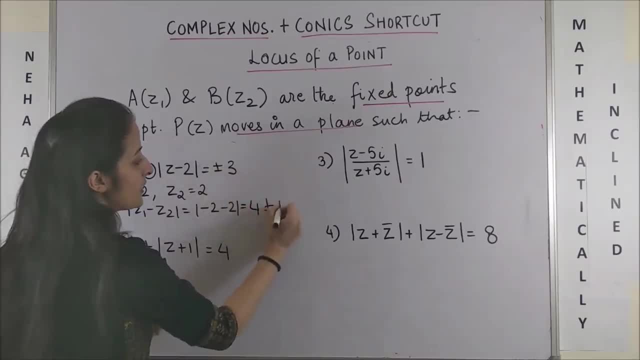 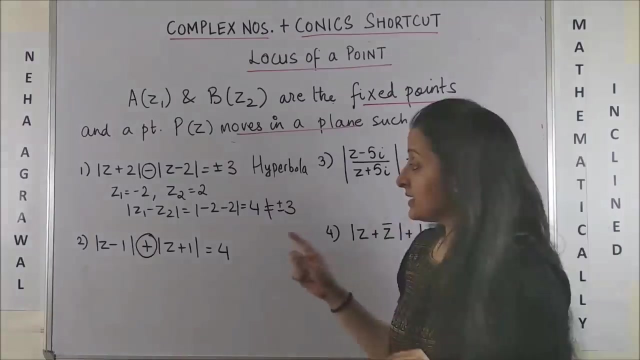 2, which is going to be a 4 and not equal to any of your plus or minus 3.. Yes, your answer was rather a hyperbola. Trust me, all these calculations you can do mentally and you can directly write. it was a hyperbola. Same way with the plus sign in between. we anticipate it to be an ellipse. Now, 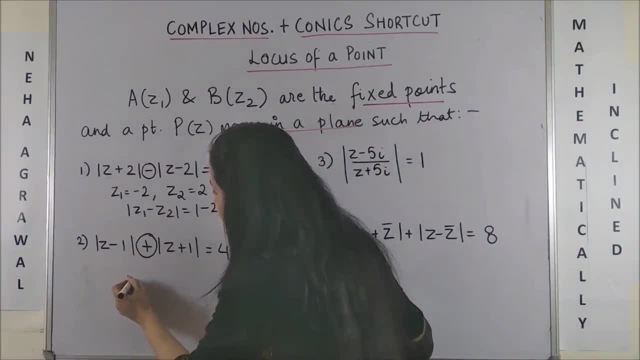 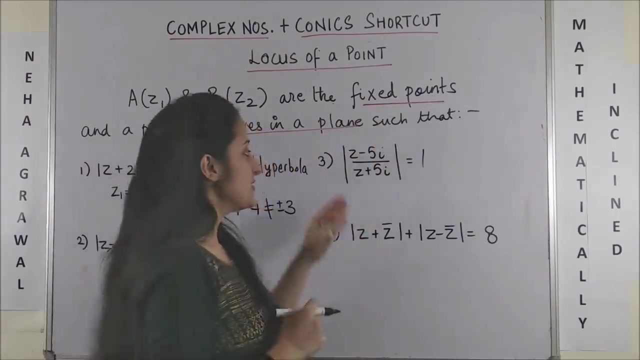 again. your z1 minus z2 would be 1 minus minus 1.. The mod turns out to be 2, which is nowhere equal to 4.. Thus the answer was a simple ellipse. Now look at the third question. You are given mod. 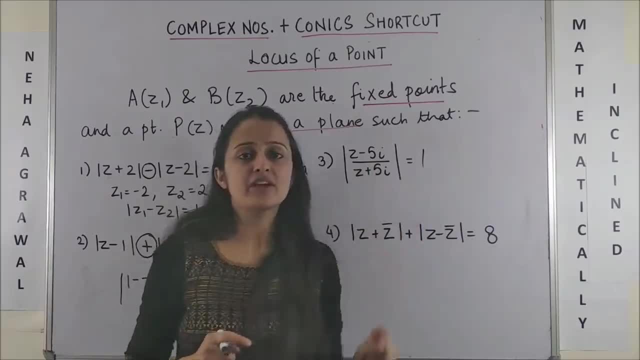 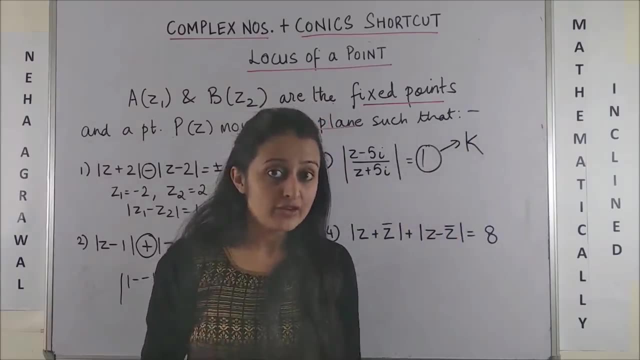 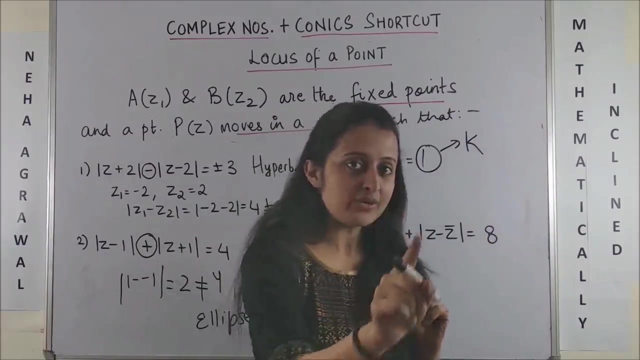 of z minus 5 iota upon mod of z plus 5 iota is equal to 1.. As you can clearly see, my k has been given as 1.. So, if you remember, if k was not equal to 1, the answer was a circle, but if k is equal to 1, in this case, the answer. 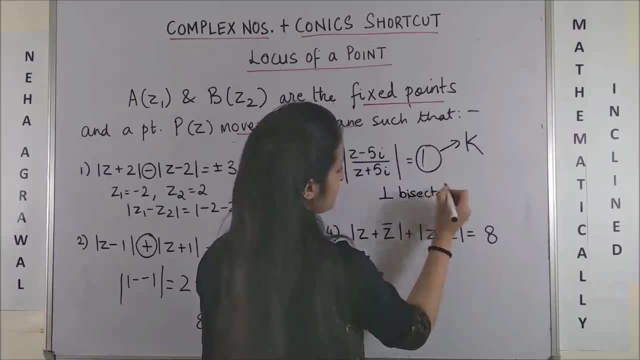 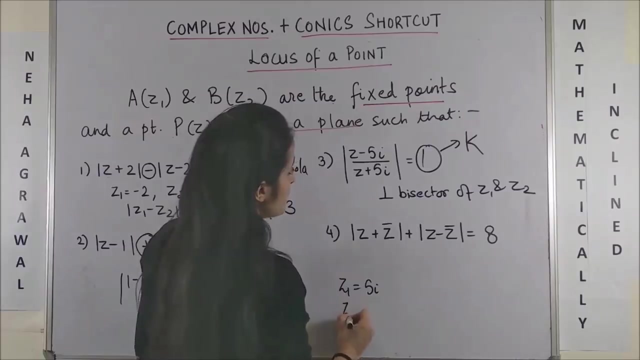 would be the perpendicular bisector. Basically, your locus P would lie on the perpendicular bisector of z1 and z2.. Now, if you realize, my z1 is 5 iota here and z2 is minus 5 iota, So they are perpendicular. 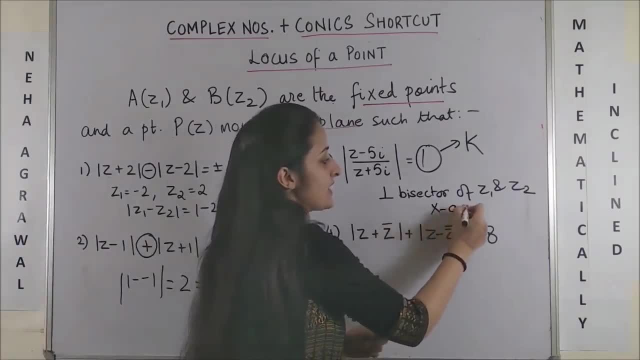 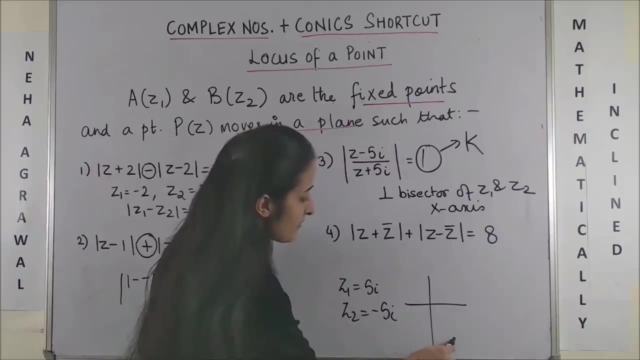 So the perpendicular bisector technically turns out to be an x axis. Why? because if you try plotting these on the plane, then what happens is: minus 5 is somewhere here, 5 is somewhere here. So their perpendicular bisector is simply your x axis. Wasn't that so quick and easy? And last but not, 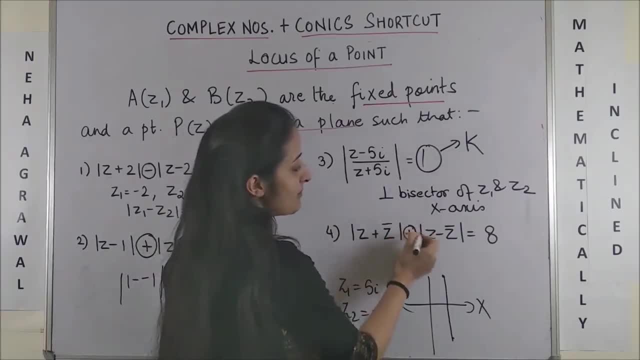 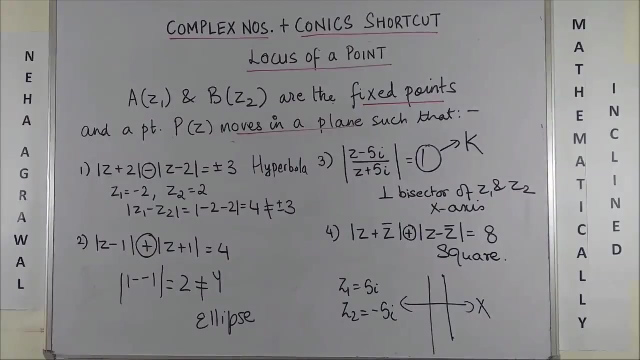 the least. our special case: z plus z bar- and there is a plus, z minus z bar is equal to 1.. So this is equal to 8.. Simply, your answer is that the locus would lie on the square. Have a look. and then we continue with more and more questions. 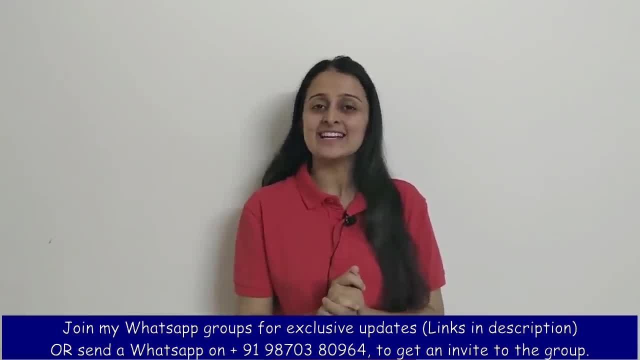 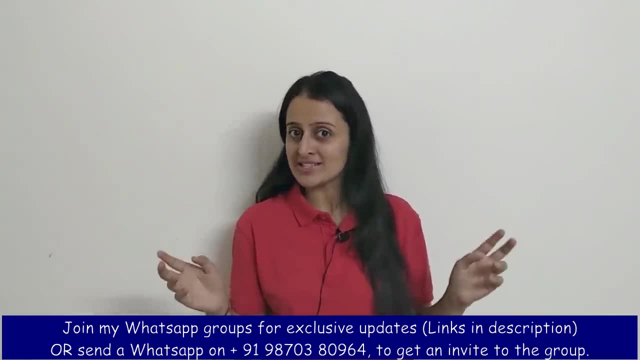 You people want to stay more and more mathematically inclined? then join my facebook page, follow me on twitter and also join me on my whatsapp group- mathematically inclined now. All the links you would find in the description box below And also for the whatsapp group. You can send me a message on this number and you would. 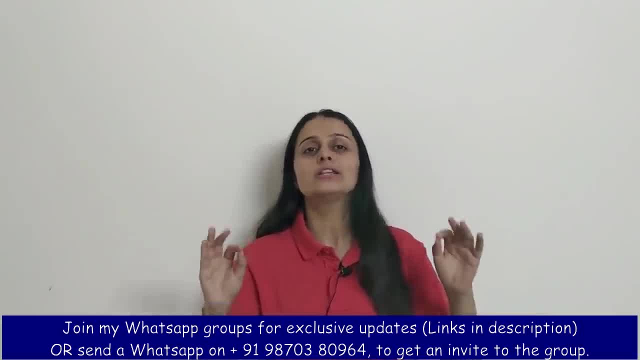 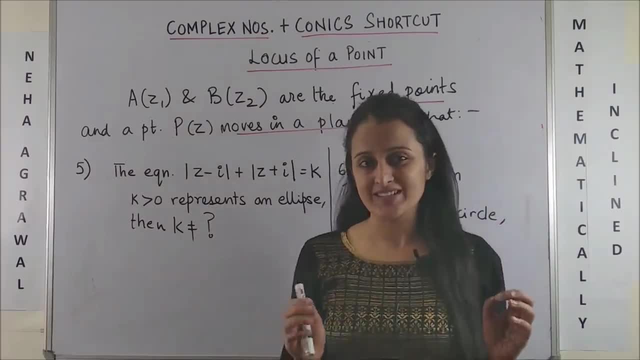 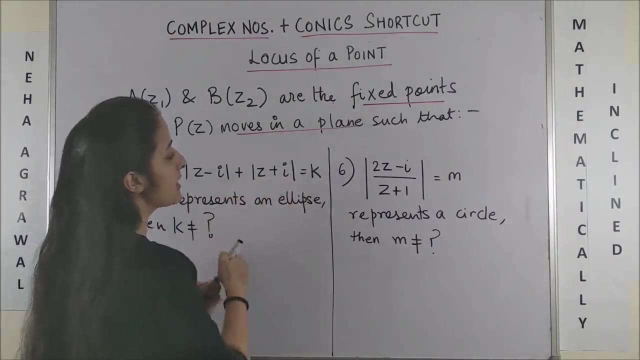 get the link. Click on that and you get all the latest updates first. And now continue watching. Coming to the next two really interesting questions, Question 5 says if the equation mod of z minus iota plus mod of z plus iota is equal to k represents an ellipse. Then 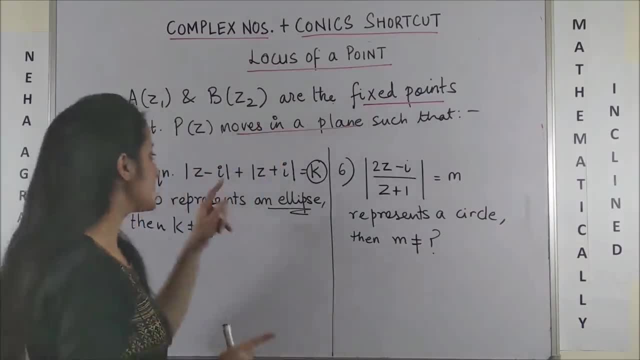 What is k not equal to? Well, you have already discussed when. if it's plus, then and it is equal to k, it cannot be an ellipse, provided your mod of z1 minus z2 is not equal to k. So here mod z1 is iota and mod z2 is minus iota should not be equal to k. So mod of or modulus of 2 iota. 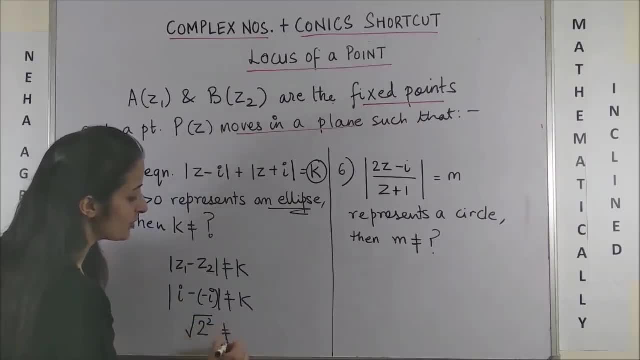 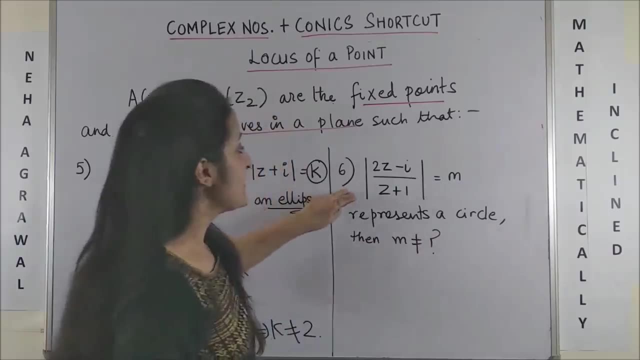 would be simply square root of 2 square, which is not equal to k. In short, k should not be equal to 2.. Same way, looking at this question, you are given that mod of this number upon this number is equal to m, then it represents a circle. then m should not be equal to what? Now, if you recollect, 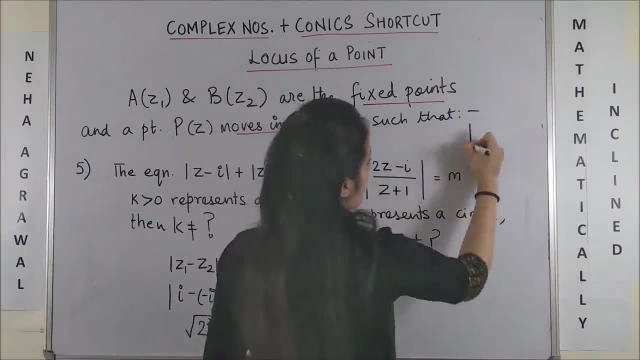 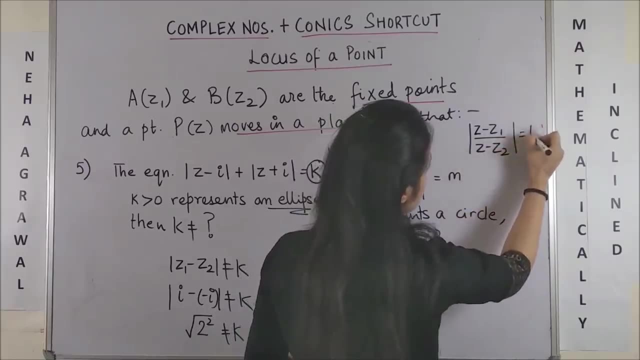 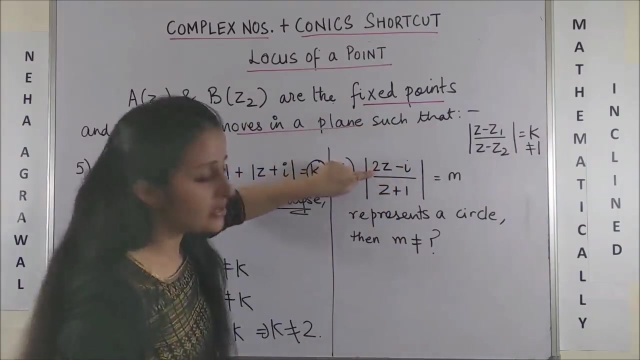 the standard form of a circle. then you know it was supposed to be: mod of z minus z1 upon mod of z minus z2 is equal to k, where k should not be equal to 1 right. But then here it is z. however, here it is twice of z. so first I have to bring this 2 outside. 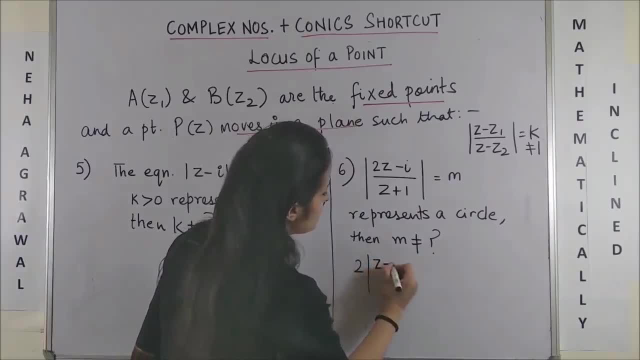 so this becomes twice of mod z minus iota by 2 upon mod of z plus 1 is equal to m. In short, if I take this m to the other side, it becomes m by 2. in short, my m by 2 is equal to k. So mod of z minus z1 upon mod of z minus iota by 2 is equal to. 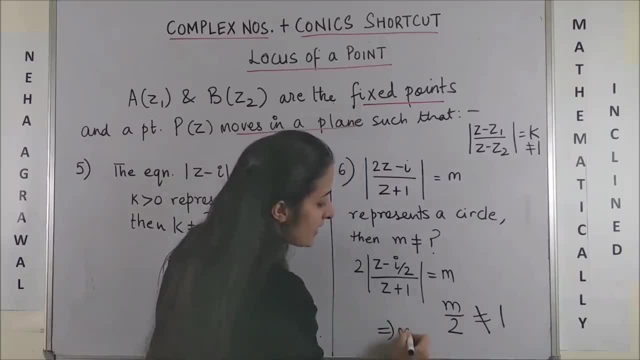 2 should not be equal to 1, or in other words, M is not equal to 2.. Wasn't this super quick? Have a look, It is time for your do it yourself. So again, A and B are given to be the fixed. 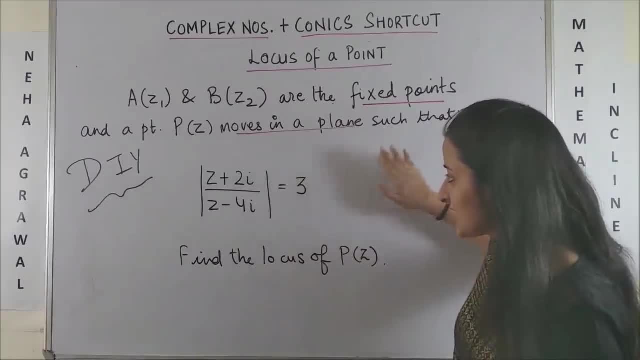 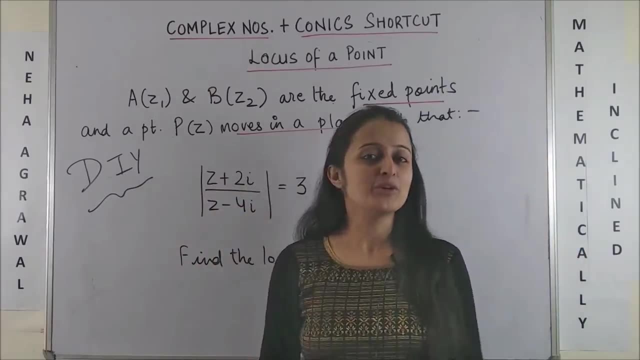 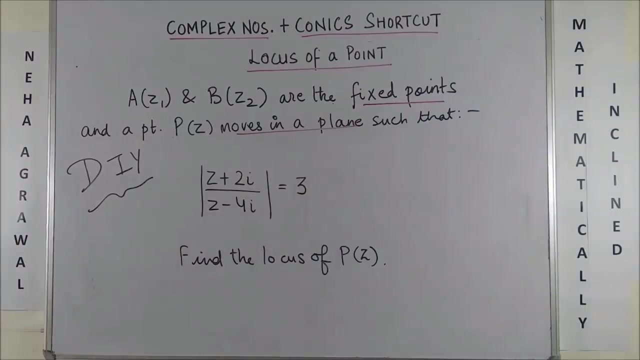 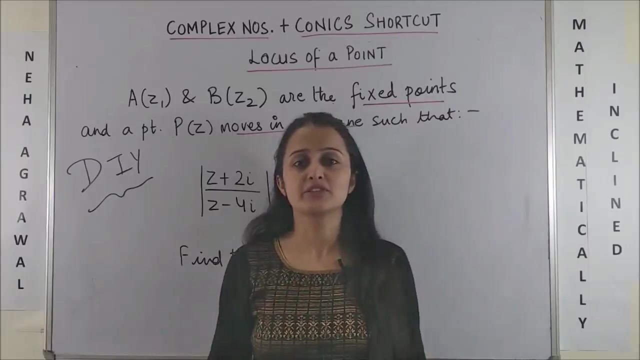 points and a point P moves in a plane such that it satisfies this equation. You have to find the locus of P Answer fast in the comment section below because you know the top 3 accurate answers always get named in my upcoming videos. I am 101% sure you people enjoyed this video. Yes, Then make sure to give this one a big. 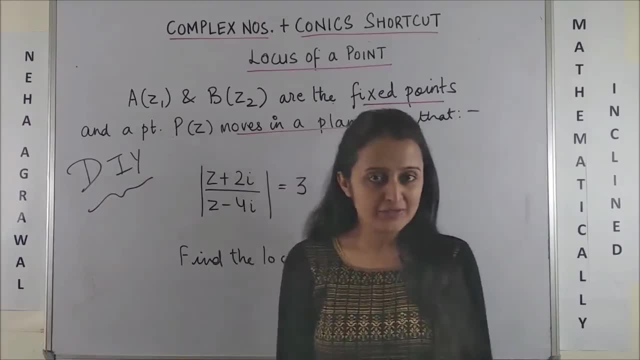 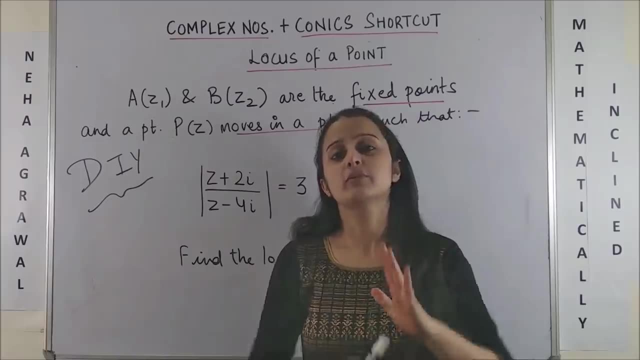 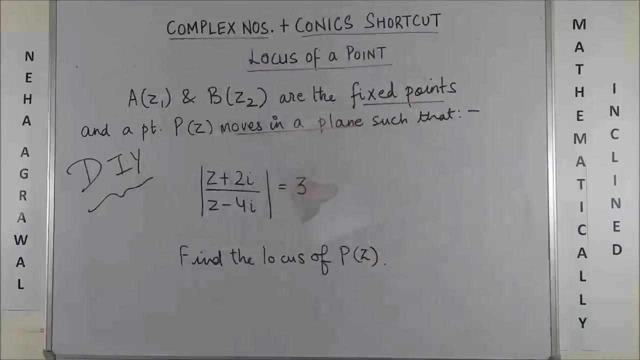 thumbs up, share it with all the people you know and, if you haven't done that so far, make sure to subscribe to my channel and hit the notification bell. I would see you with a lot of new and exciting videos very, very soon. Until then, bye, bye.